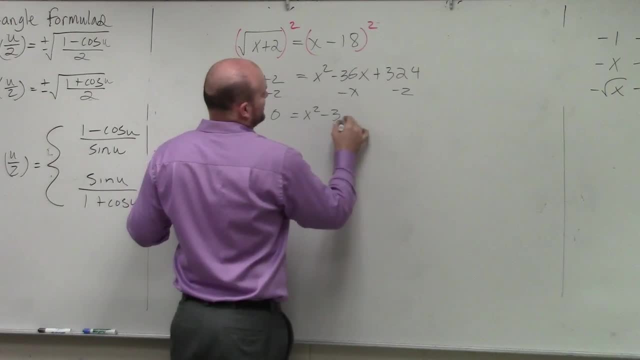 So I have 0 equals x squared minus 36x plus 322.. 37.. 37,. thank you, I forgot to do that. All right, So we'll look at this problem and we'll say, ooh, this does not look like fun to factor right. 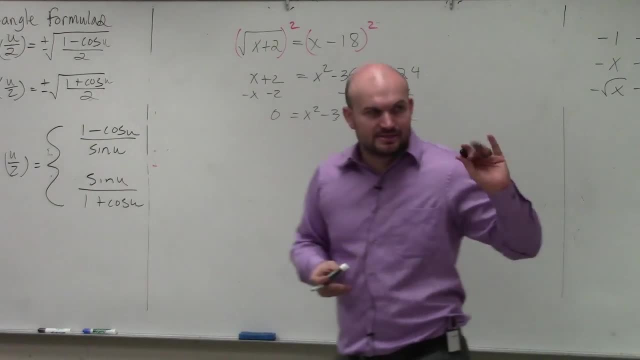 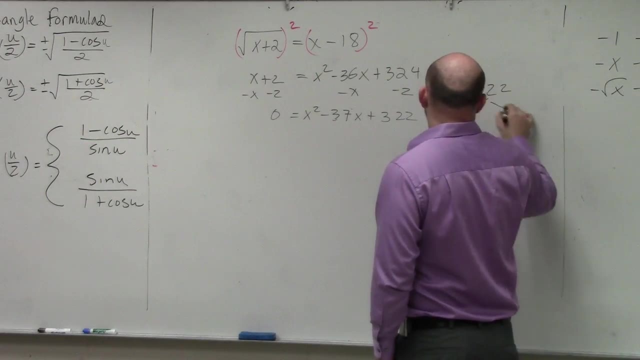 Well, So the main important thing when factoring this is: I would just start listing out the factors and see where we get And I don't. so if I have 322, the first factor would be 322 times 1.. 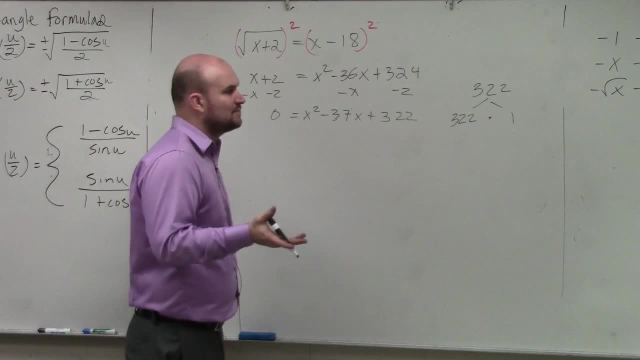 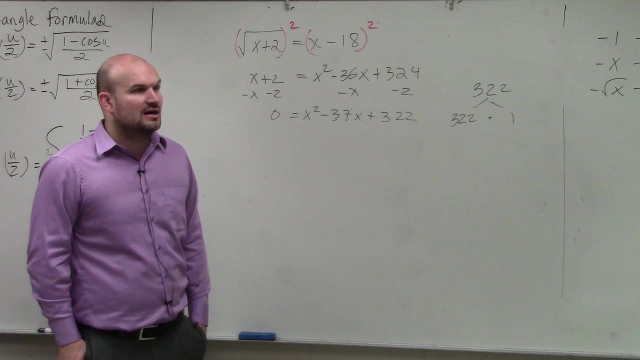 And I always start with my largest, you know factor: 322 times 1.. Then I'd say, well, what about 2?? I know 2 divides into this right. 2 would divide into that 161.. 161.. 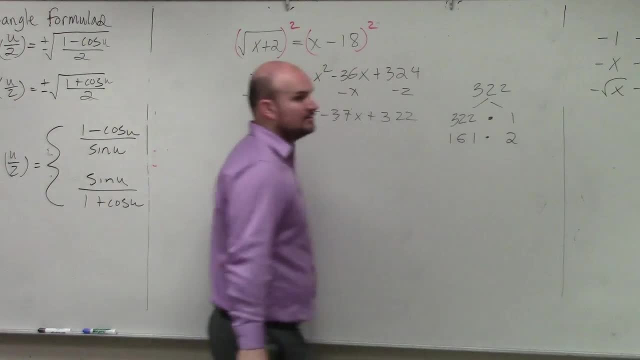 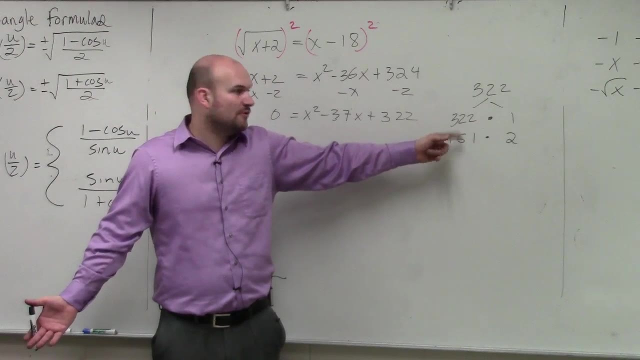 That was going to be way down the line, But all right. Well, can I divide 161 divided by 2? again, Yeah, No, you can't. So therefore, I know it's not divisible by 4.. What about divisible by 3?? 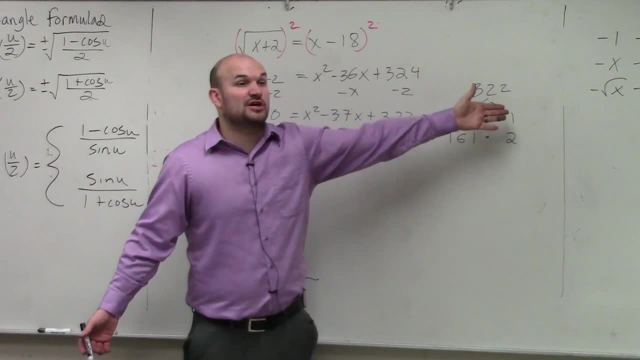 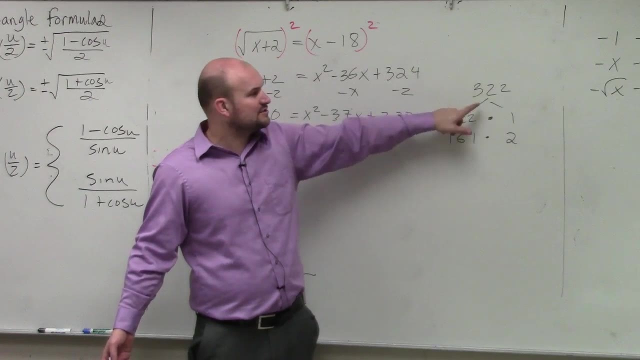 Does 3 divide into that? No, No, 4 doesn't go. We know 5 doesn't go right. Is 6 divisible? Nope, 6 isn't divisible. 7, I don't believe there's anything. yeah, 42, so it could be. 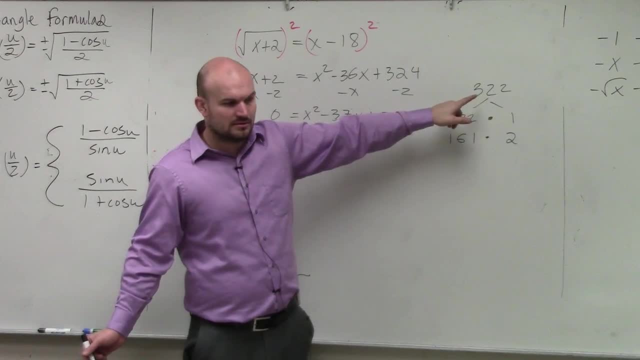 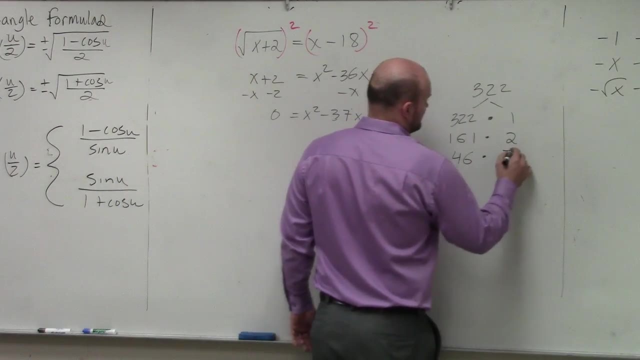 7 divisible. Yeah, it could be. Yeah, How many times? Yeah, yeah, 46 times 46.. So I have 42.. Yeah, 46 times 7.. What about 8?? No, 9?. 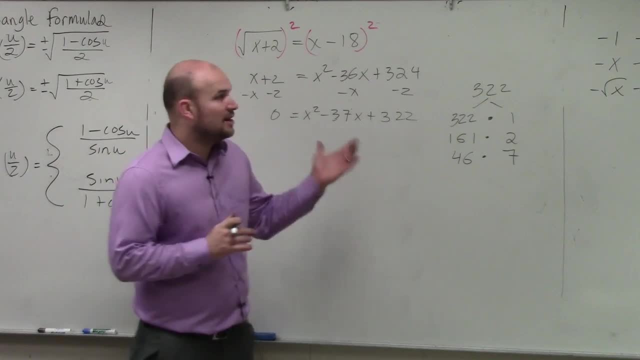 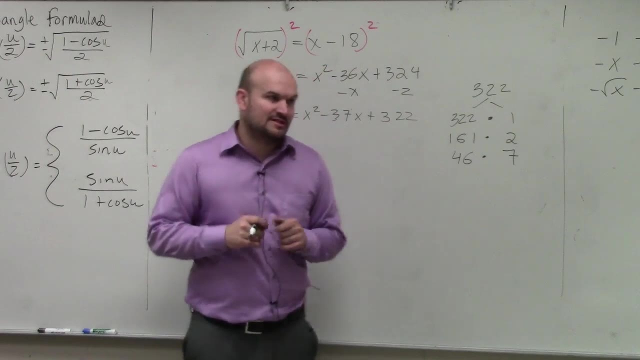 Yeah, I can say that No 10,, we know No 11,, no No 12. 13. Yeah, 14. 13,, 14.. So what's 14?? 14.. 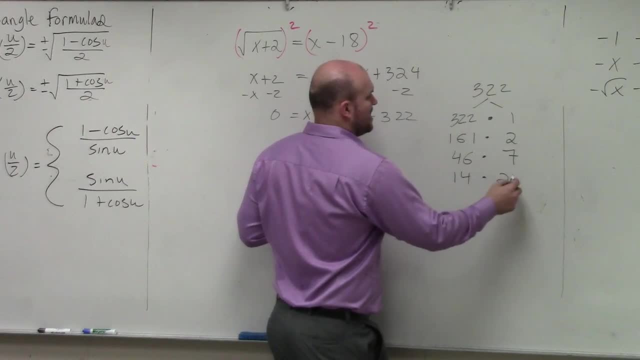 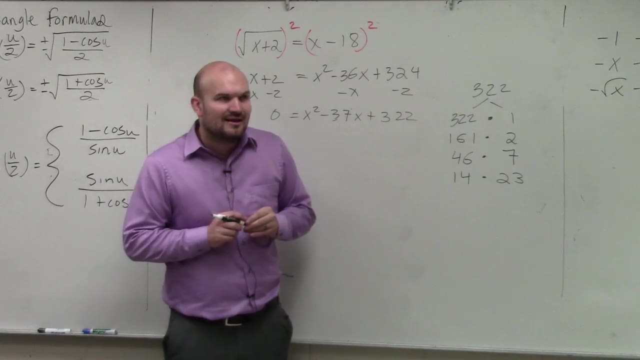 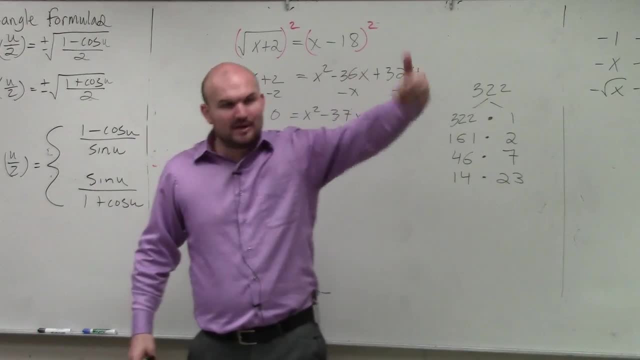 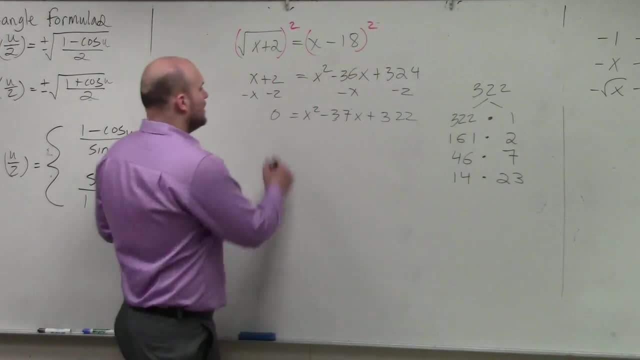 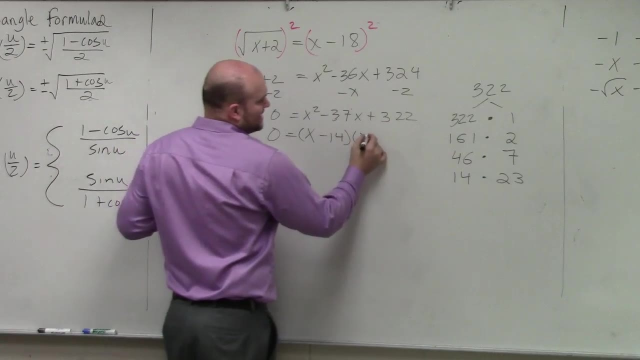 Right, Start at 1 and then keep on going. So now I can factor this to x. I know that they both have to be negative, Minus 14 times x minus 23.. Now I apply the zero product property.